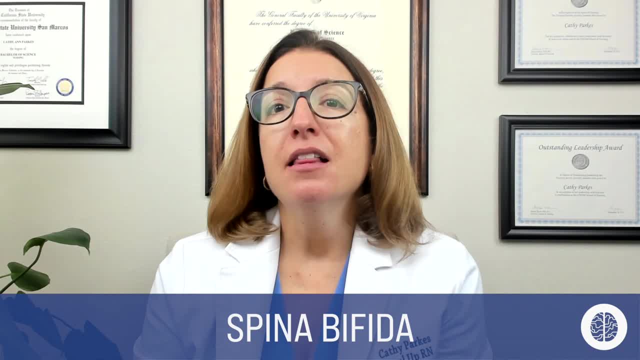 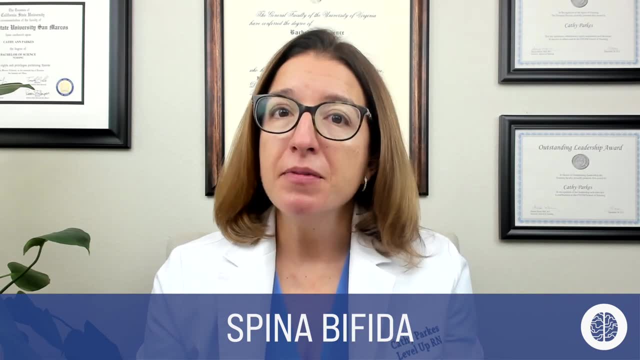 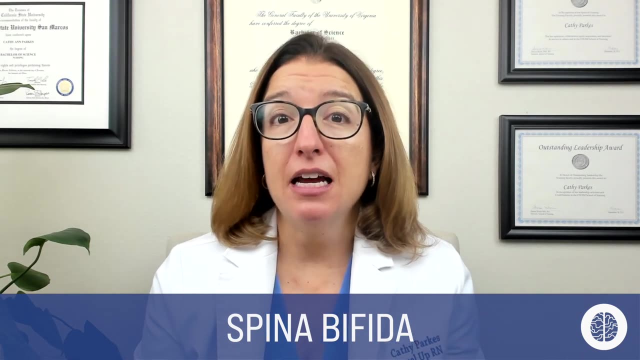 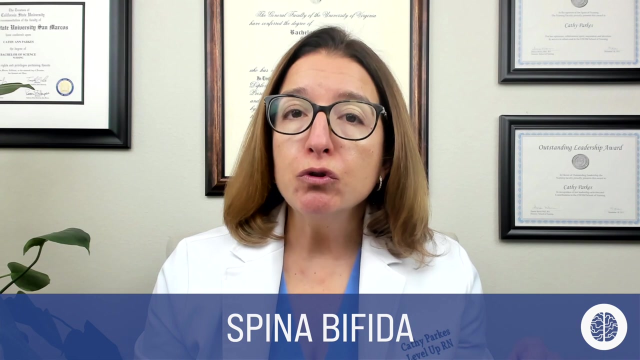 First we have spina bifida occulta. This is where we actually can't see the malformation in the spinal cord because skin is covered. The second type of spina bifida is called meningocel. This is where we have a protrusion. 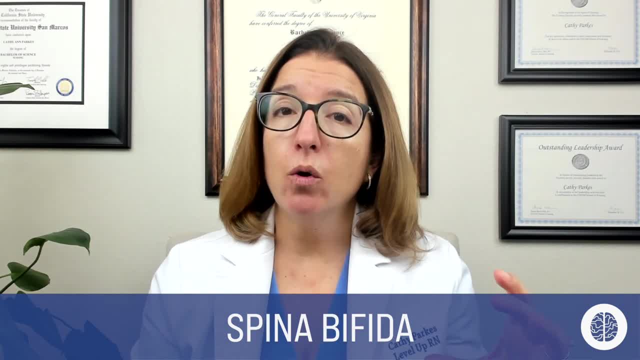 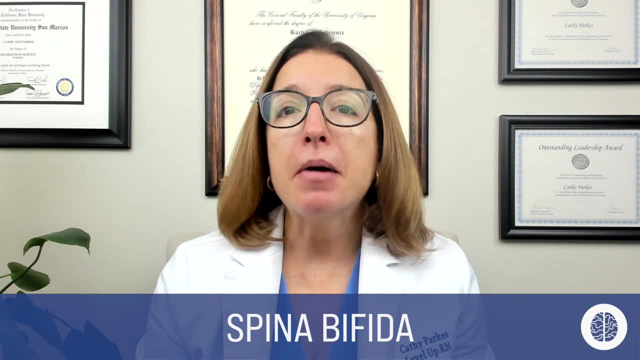 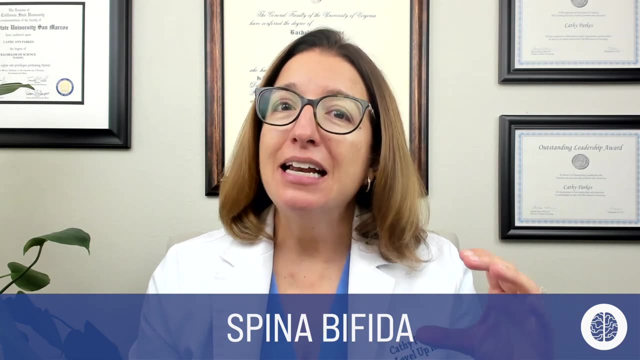 of a sac or a cyst over the baby's spinal cord that contains cerebral spinal fluid as well as meninges. And then, lastly, we have myelomeningocel. This is where we have a protrusion of a sac or cyst over the spinal cord, And in that sac we have cerebral spinal fluid, meninges. 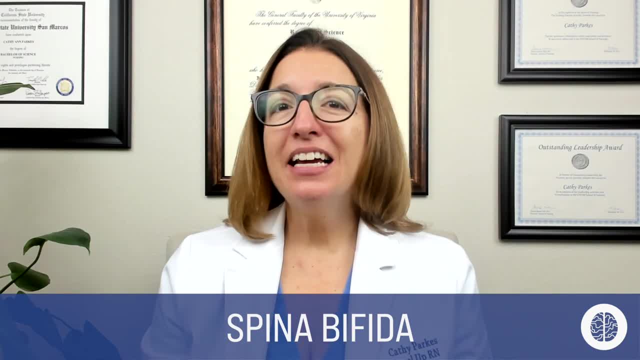 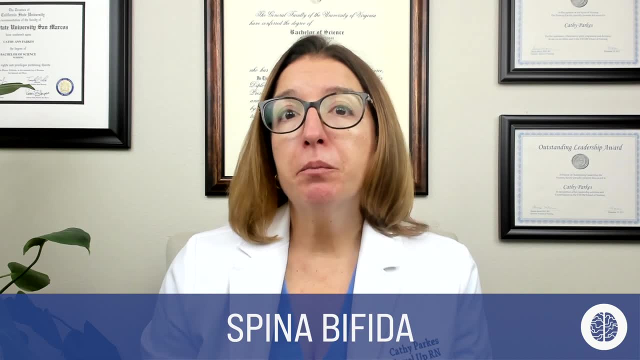 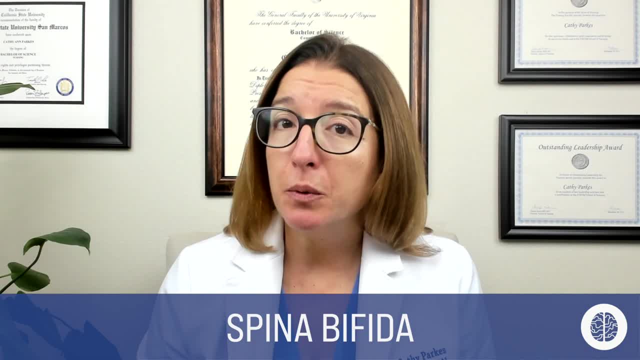 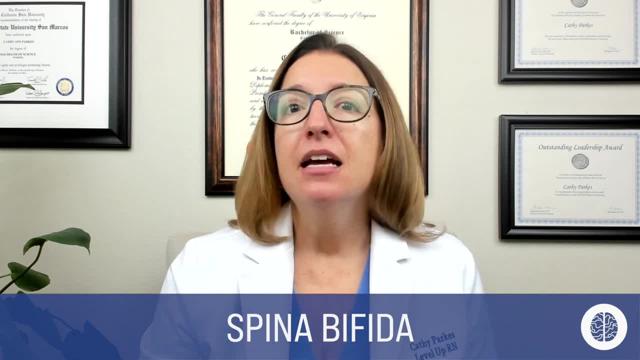 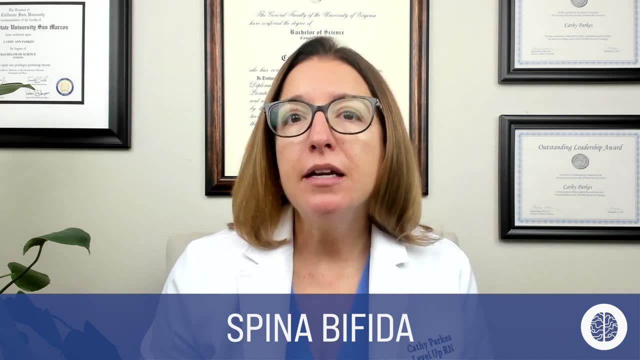 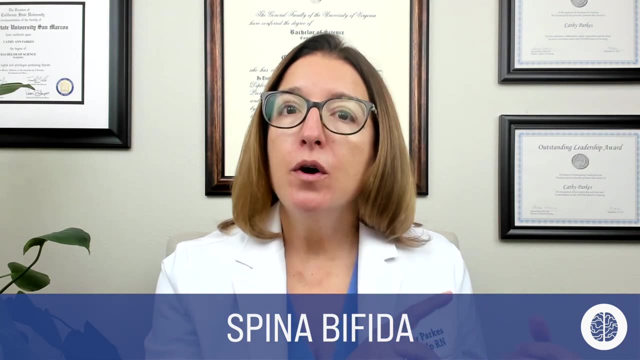 is discovered during the prenatal period. In terms of nursing care, if the baby is born with a meningocel or myelomeningocel, we need to protect that protruding sac. So we're going to want to cover that sac with a sterile, saline-moistened, non-adherent dressing And we want to 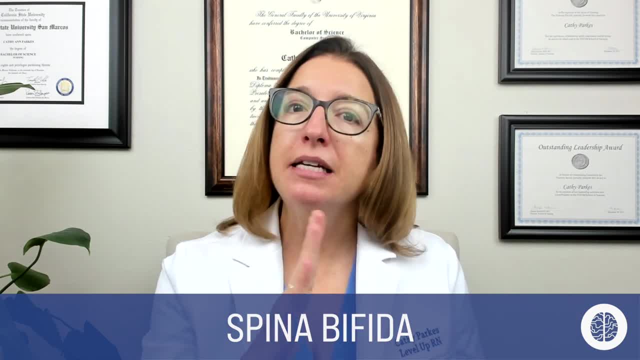 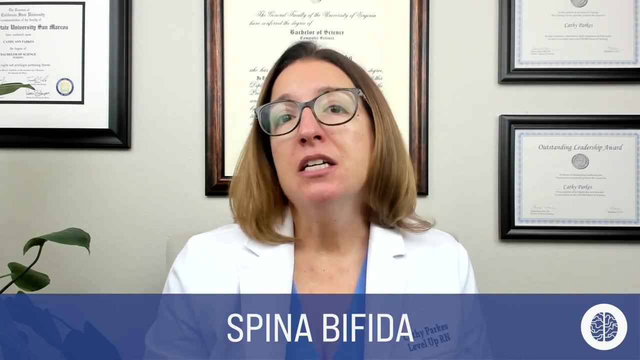 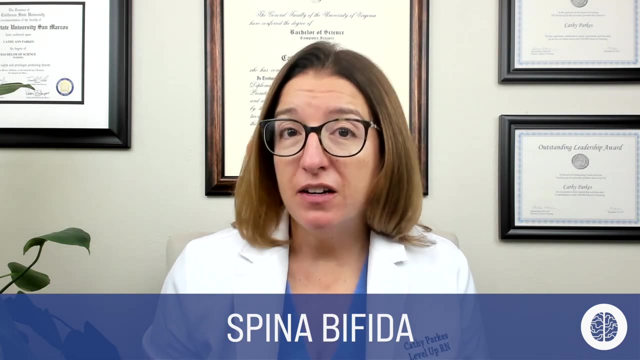 avoid any kind of pressure to that sac, So we're going to place the baby in a prone position, so tummy side down with their hips flexed. We also need to provide some important teaching to the family regarding complications that can occur with spina bifida, which includes 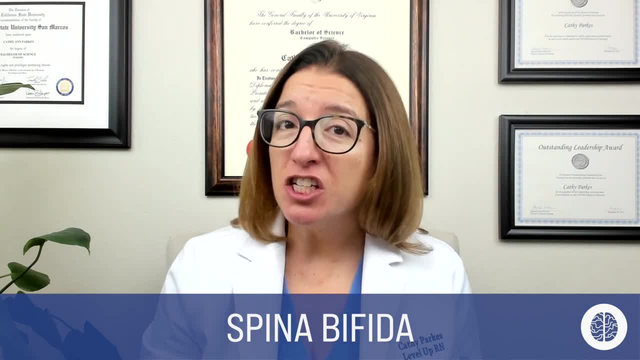 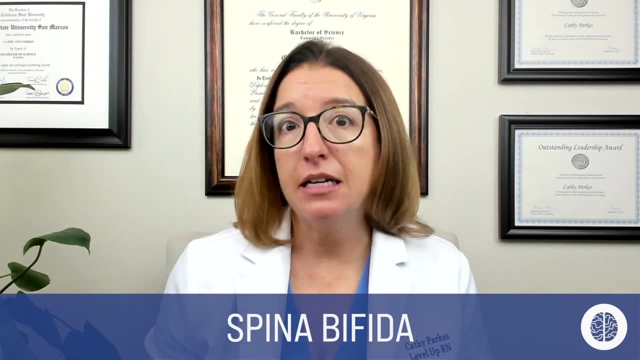 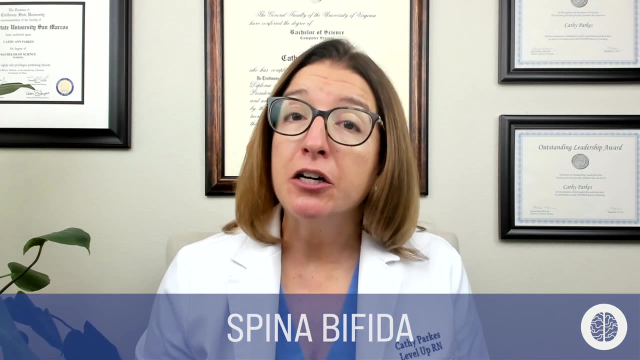 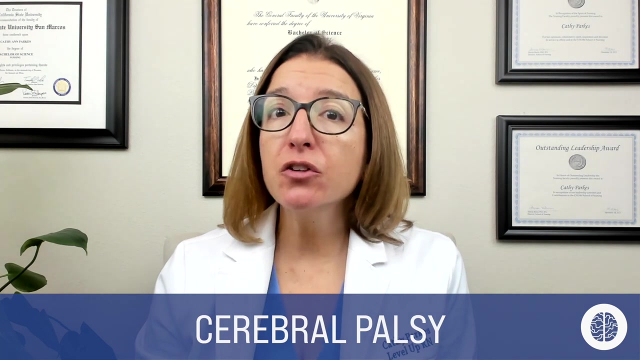 hydrocephalus, as well as latex allergies. The child will likely have an increased risk for pressure injuries, as well as burns, which relates to their lack of sensation, And then bladder dysfunction is also common that often requires intermittent catheterization. Next, I want to briefly talk about cerebral palsy, which is a neurological 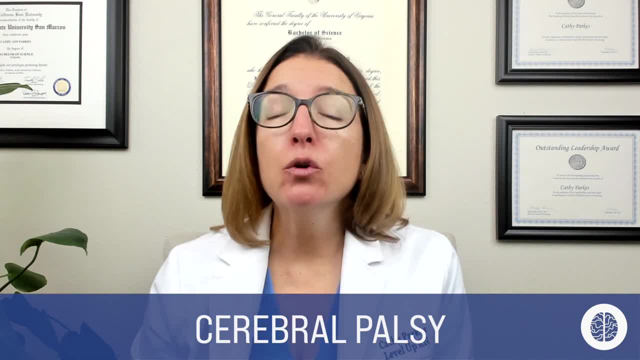 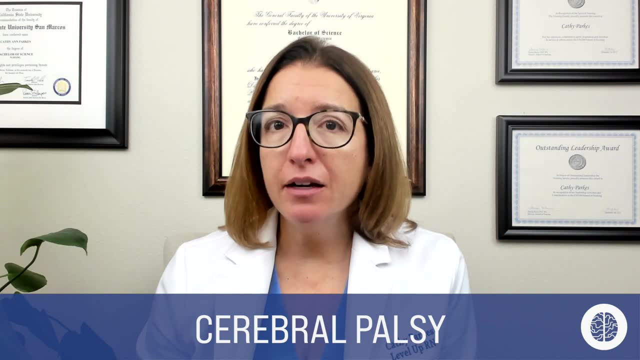 disorder that affects body movement and muscle coordination. So with this disorder we have abnormal intrauterine development of the brain or some kind of hypoxic brain injury that damages the cerebral cortex and the brain. And then we want to talk about cerebral palsy, which is a neurological 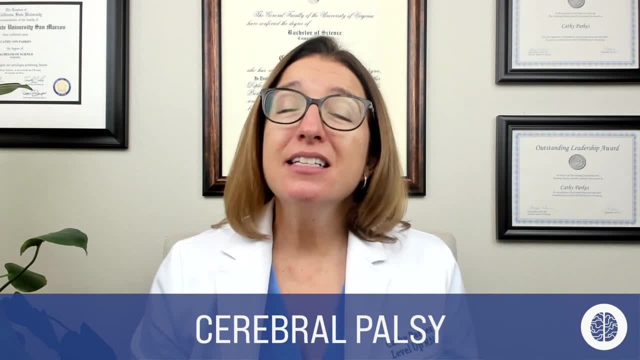 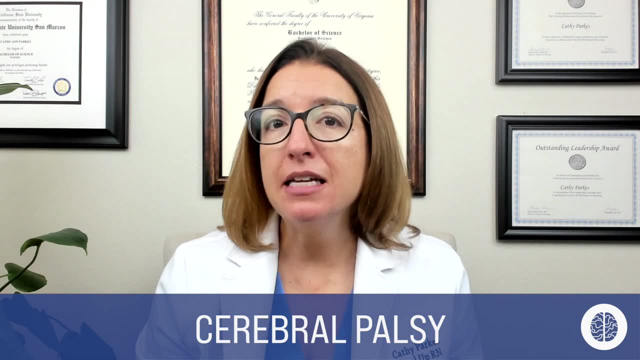 disorder that affects the brain. So we're going to talk about cerebral palsy, which is a neurological disorder that affects the cerebral cortex and affects motor function. So signs and symptoms will include ataxia, so lack of coordination, as well as muscle spasticity and impaired gait. 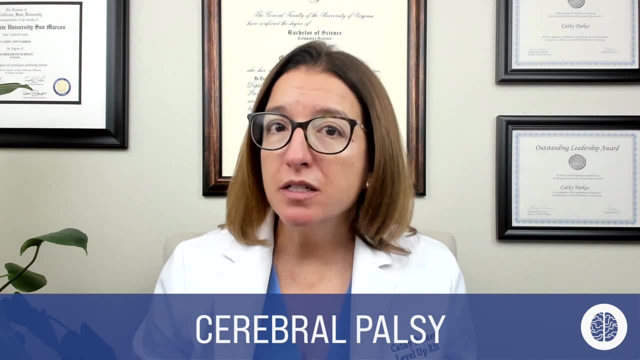 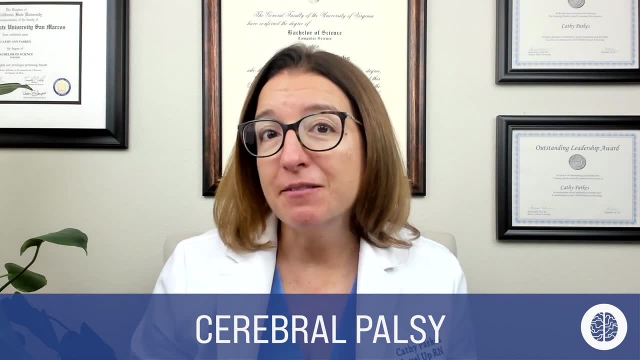 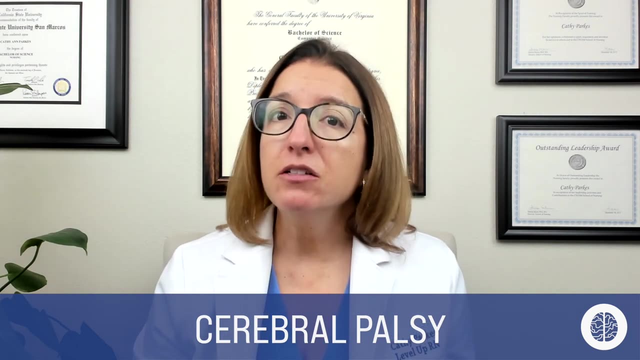 In severe cases, we can have intellectual disability and seizures, as well as impaired swallowing, speech, vision and hearing. In terms of treatment, we can actually use Botox or interfecal baclofen. In terms of treatment, we can actually use Botox or interfecal baclofen to address the muscle spasticity. 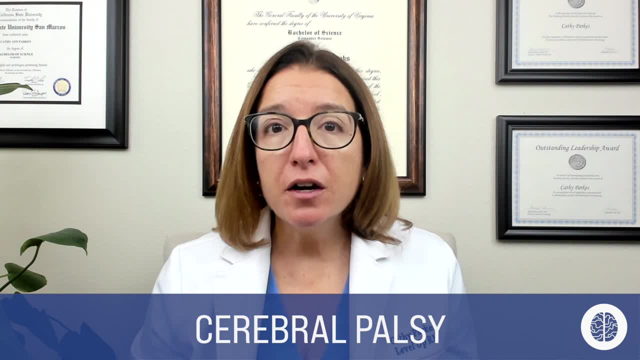 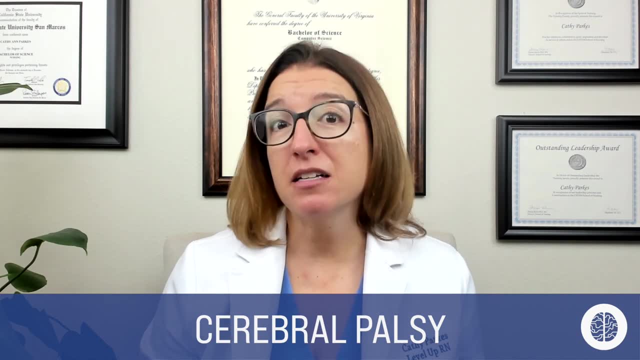 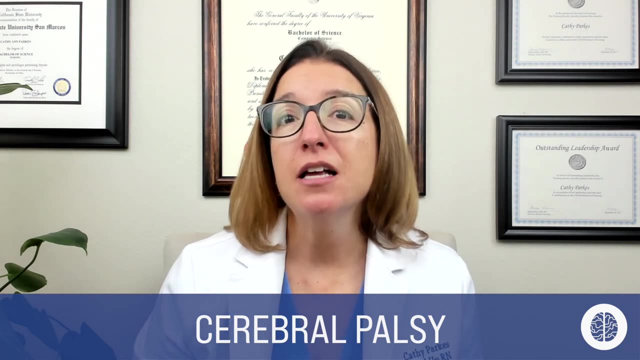 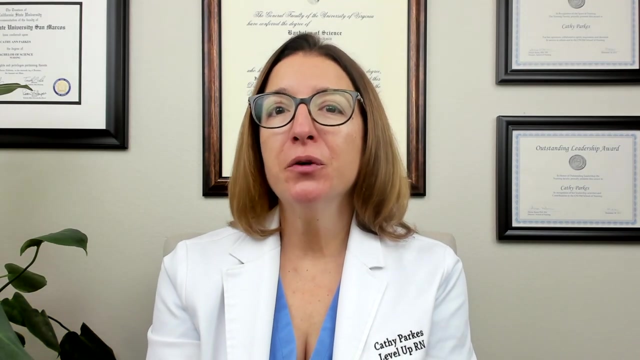 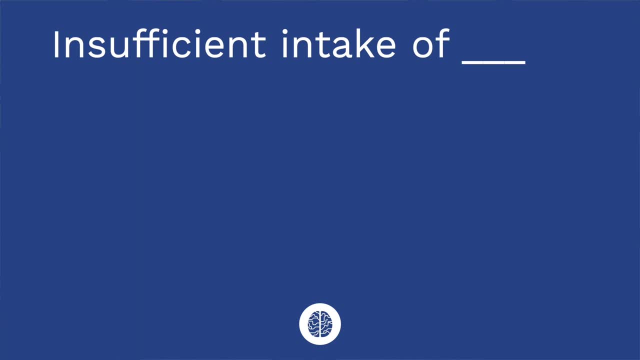 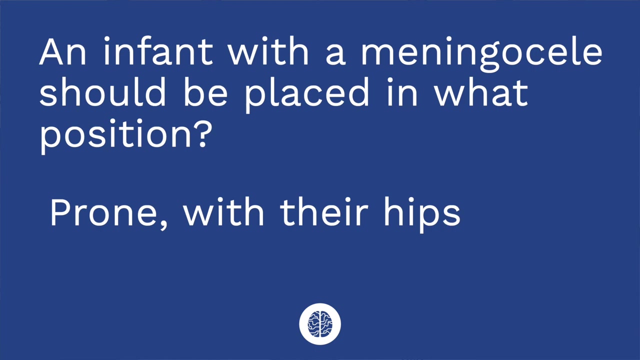 Question: Insufficient intake of blank during pregnancy increases the risk for spina bifida? The answer is folic acid. Question number two: an infant with a meningecele should be placed in what position? The answer is prone with their hips flexed. Question number three: 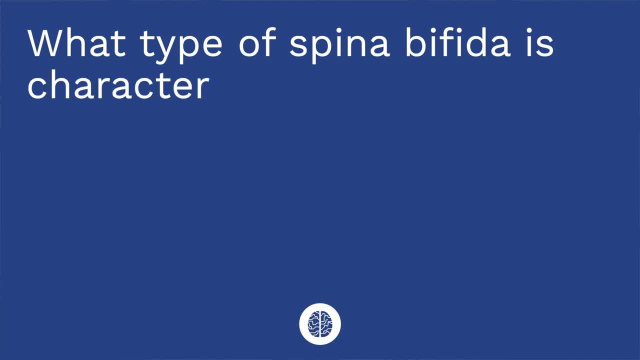 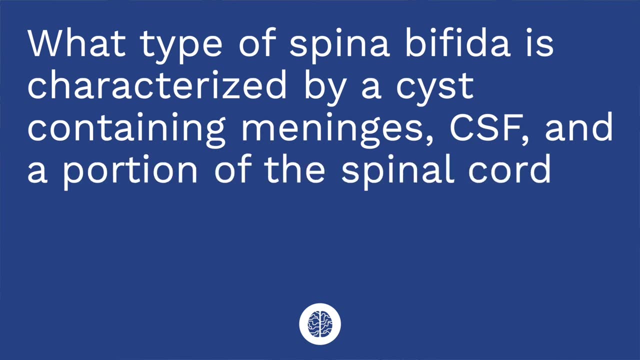 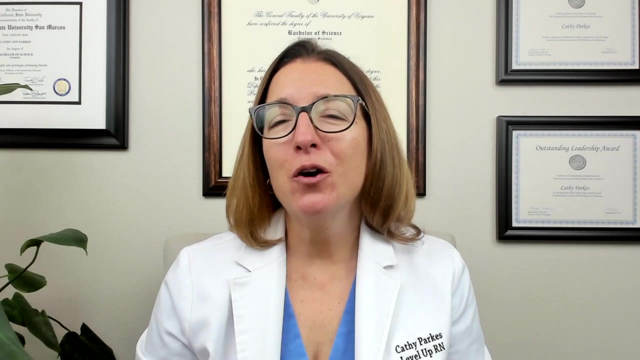 what type of spina bifida is characterized by the protrusion of a cyst with meninges, cerebral spinal fluid and a portion of the spinal cord? The answer is myelomeningocele. All right, I hope we did well on that quiz.